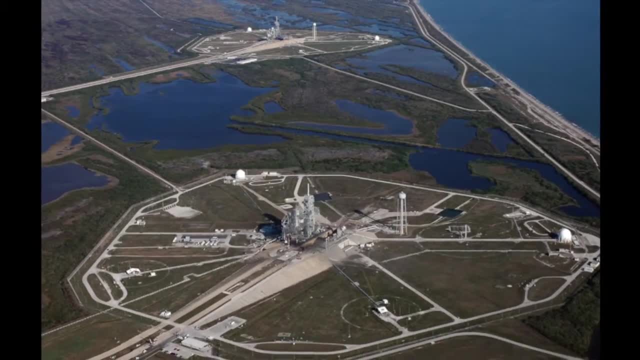 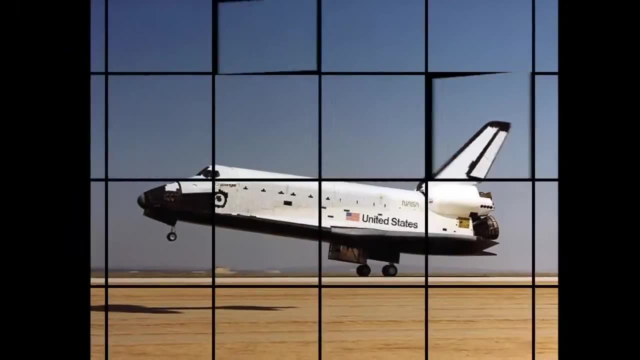 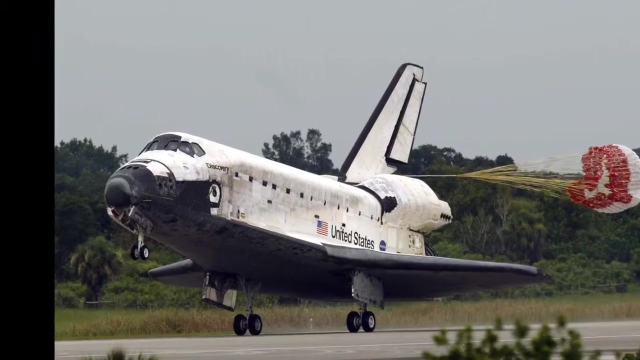 for this shuttle, and it is Complex 39, pads A and B. The Space Shuttle became the major focus of NASA in the late 1970s and 80s. planned as a frequently launchable and mostly reusable vehicle, Five Space Shuttle orbiters were. 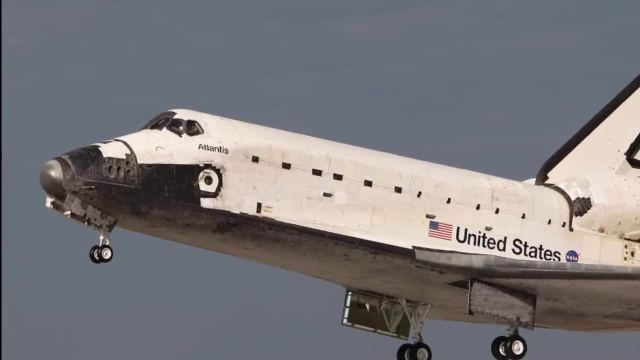 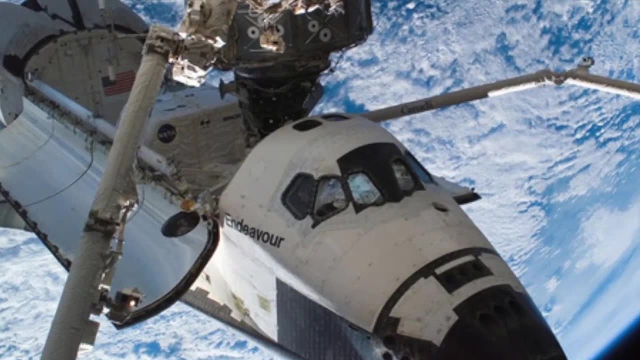 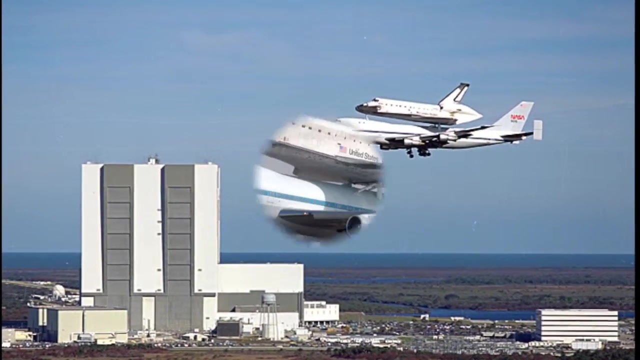 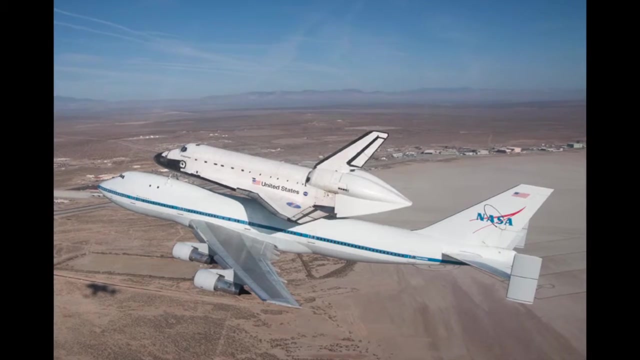 built by 1985.. The first to launch was Columbia on April 12, 1981, following the launch of Challenger Discovery. Atlantis and Endeavour, The Shuttle Carrier Aircraft SCA, were two extensively modified Boeing 747 airliners that NASA used to transport space shuttle. 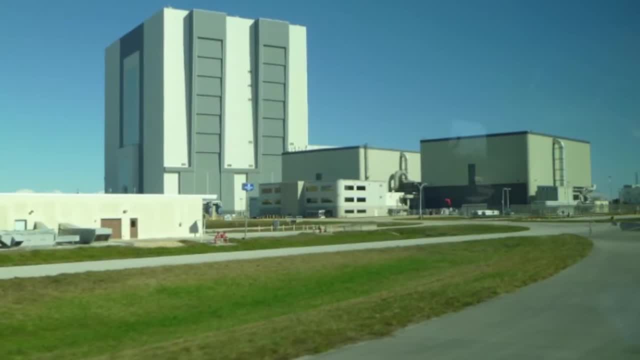 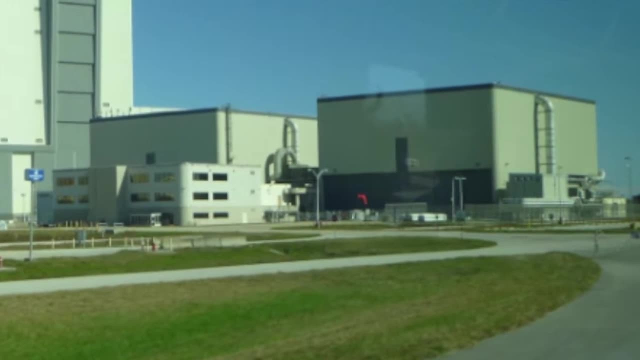 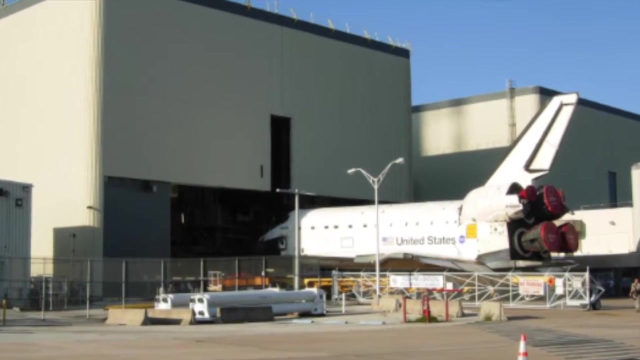 orbiters. The Orbiter Processing Facilities, or OPS, were one of three hangars like a custom-made garage for the orbiters. This is where they underwent maintenance between flights. All three OPS were located at the NASA Kennedy Space Center in the Launch Complex 39.. 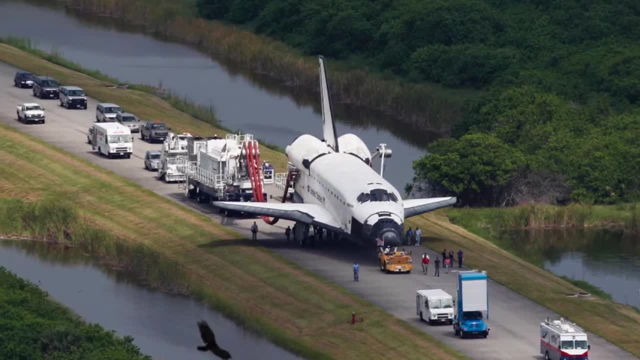 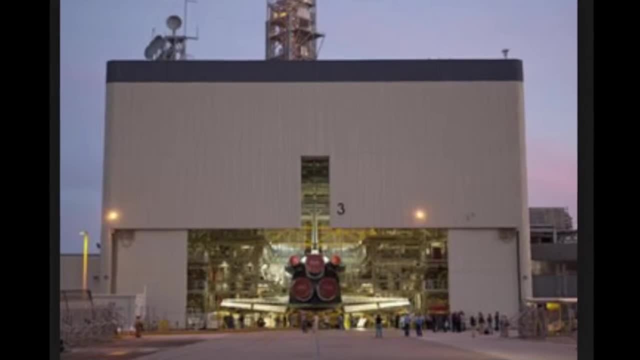 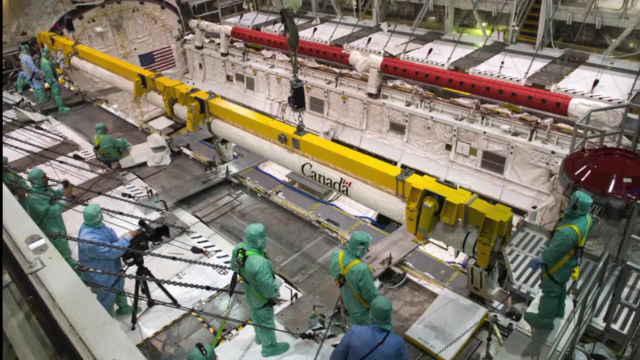 When the shuttle mission was completed, the orbiter was towed from the Shuttle Landing Facility to its assigned OPF, where it spent several months- typically less than 100 days, being prepared for the next mission. Any remaining payload from the previous missions were removed. 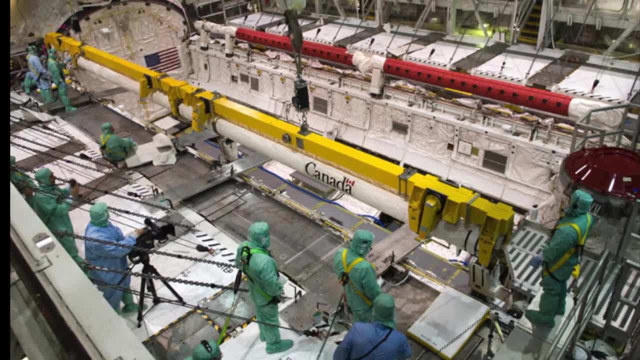 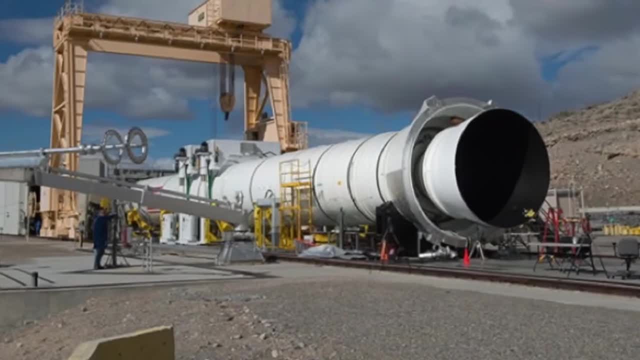 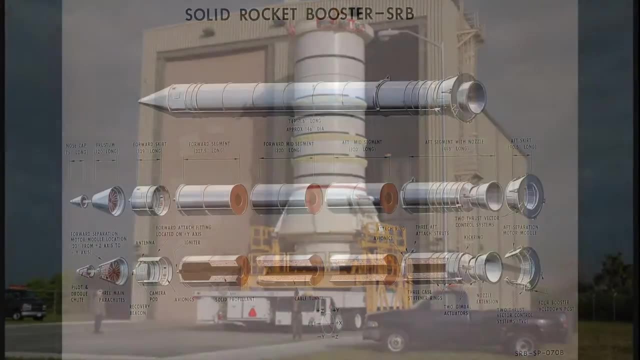 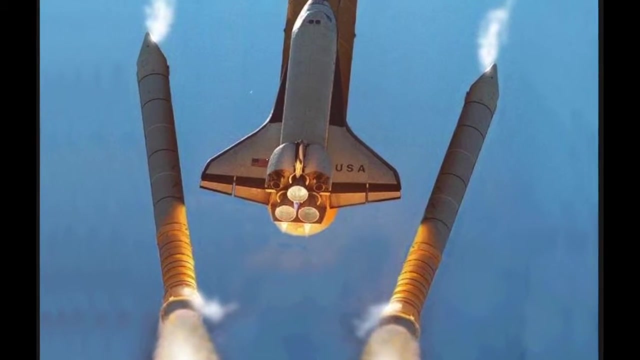 and the vehicle was fully inspected, tested and refurbished. The Space Shuttle Solid Rocket Boosters, or SRBs, were the first solid-fuel motors to be used for primary propulsion on a vehicle used for human spaceflight. It provided the majority of the space shuttle's thrust during the first two minutes of flight After burnout. 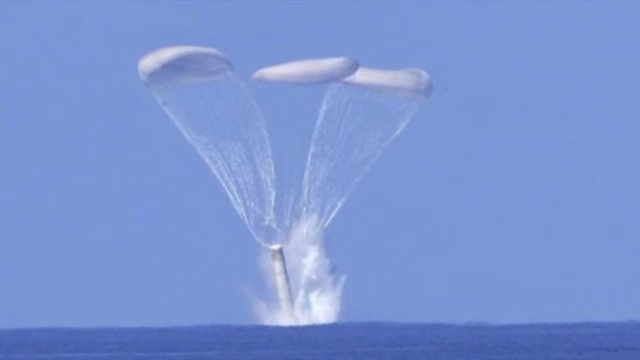 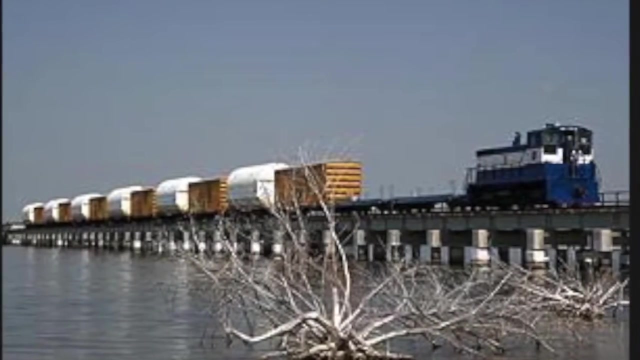 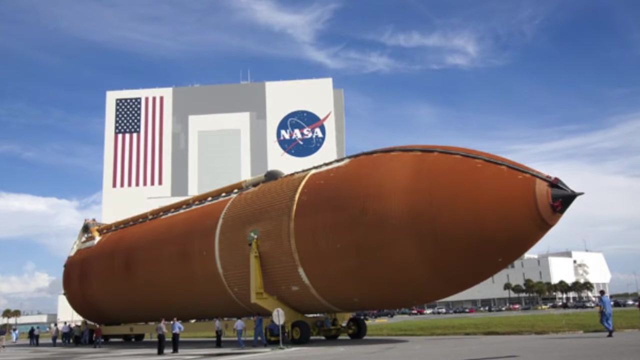 they were jettisoned and parachuted into the Atlantic Ocean, where they were recovered, examined, refurbished and reused. The rocket fuel was manufactured in Utah and brought in on a train. A Space Shuttle external tank was the component of the Space Shuttle launch vehicle. 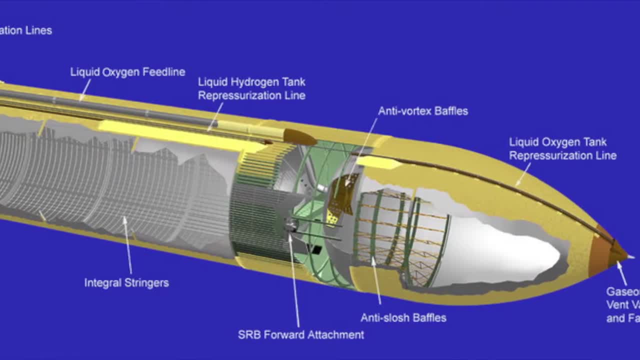 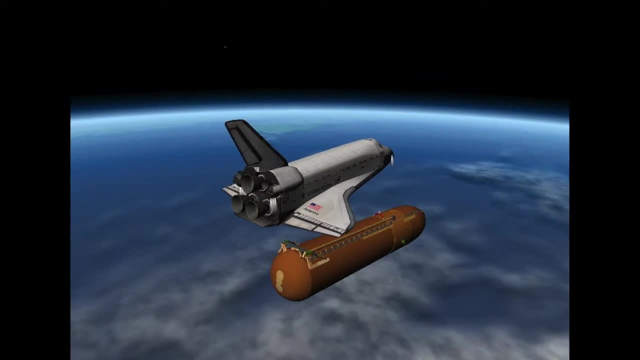 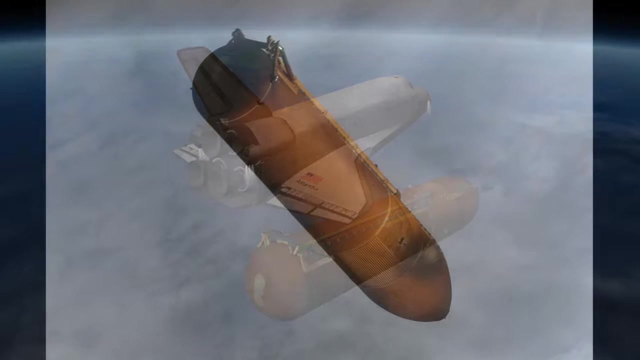 that contained the liquid hydrogen fuel and liquid oxygen oxidizer. During lift-off and ascent it supplied the fuel and oxidizer under pressure to three space shuttle main engines in the orbit. It escaped from various stations for production, including the mission. The ET was ejected just over 10 seconds after MECO or Main Engine Cut-Off. 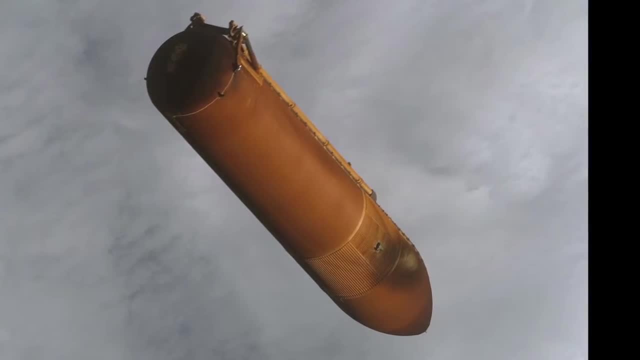 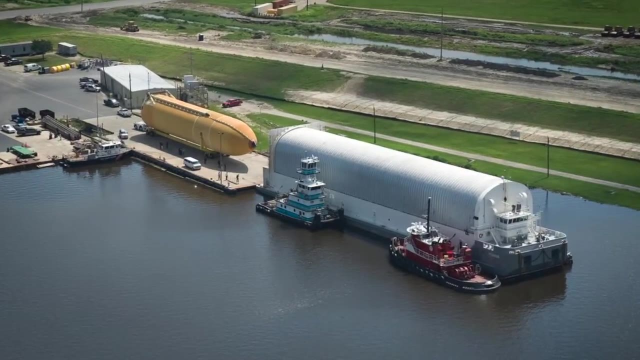 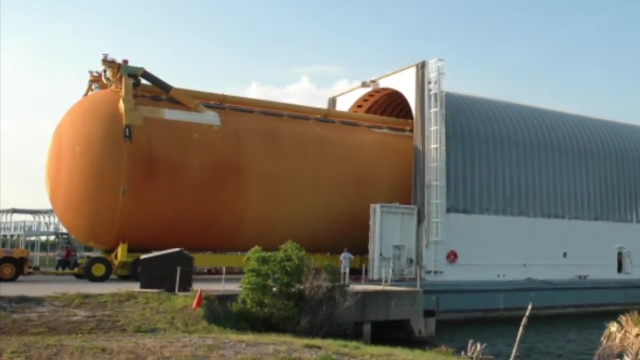 Unlike the solid rocket boosters, external tanks were not reused. They broke up, entering the atmosphere before impact in the ocean and were not recovered. The contractor for the external tank was Lockheed Martin. The tank was manufactured in New Orleans, Louisiana, and was transported to Kennedy Space. 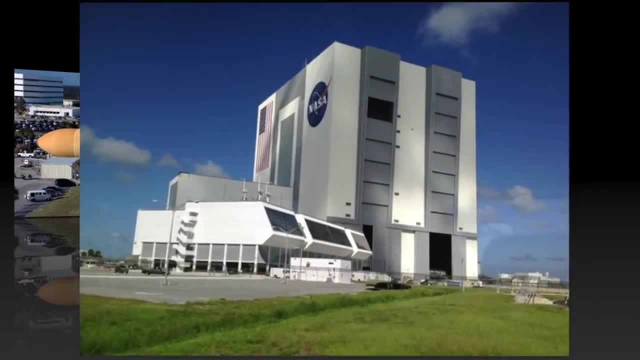 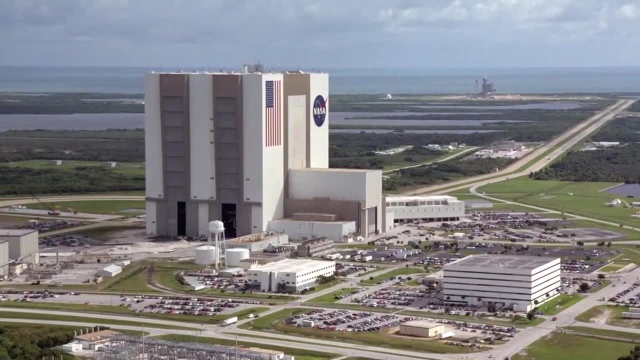 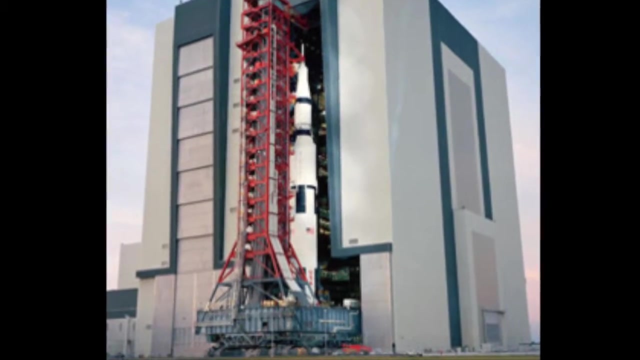 Center by barge. The Vehicle Assembly Building, or the VAB, was designed to assemble large space vehicles. It was originally built in 1966 to allow for the vertical assembly of the Saturn V rocket. The building covers 8 acres and encloses almost 130 million cubic feet of space. 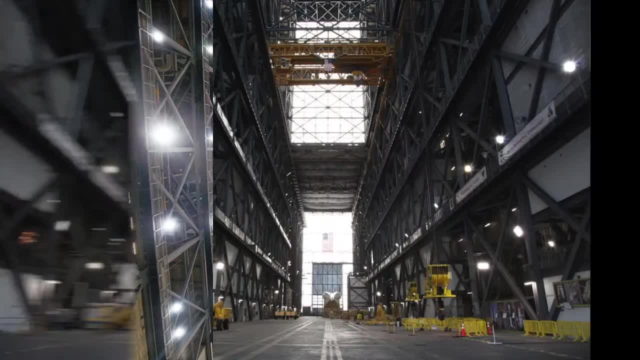 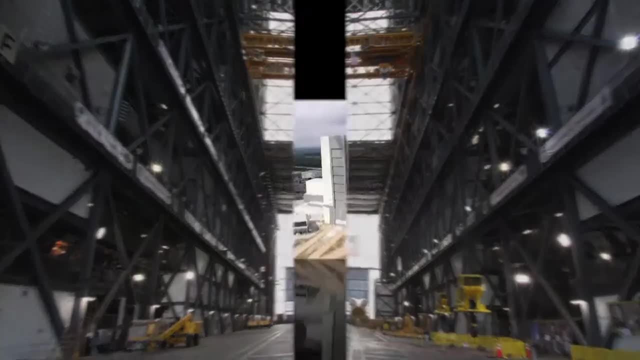 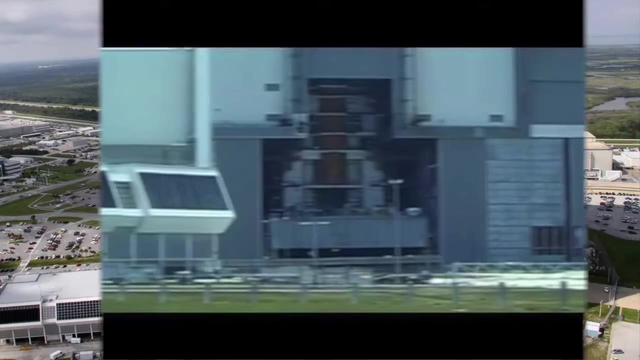 There are four bays located inside the building, which are the four largest doors in the world. Each door is 456 feet high, It has seven vertical panels and four horizontal panels, and it takes 45 minutes for the doors to completely open or close. 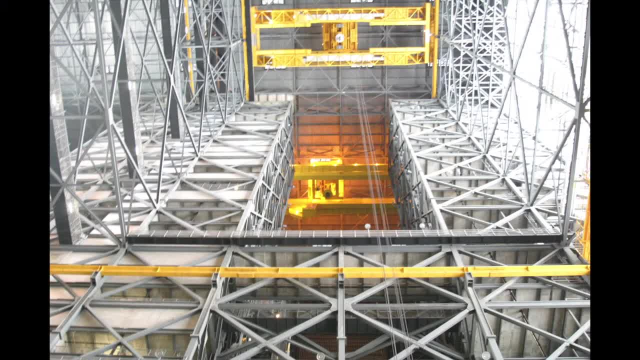 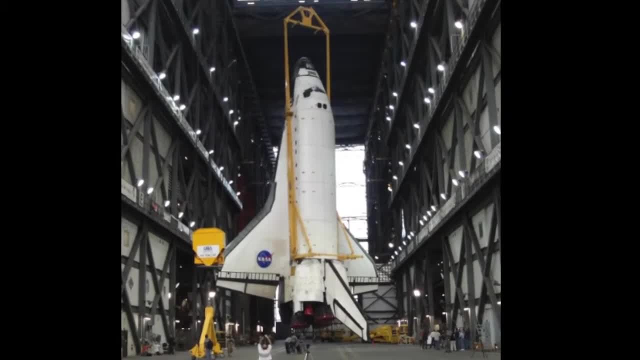 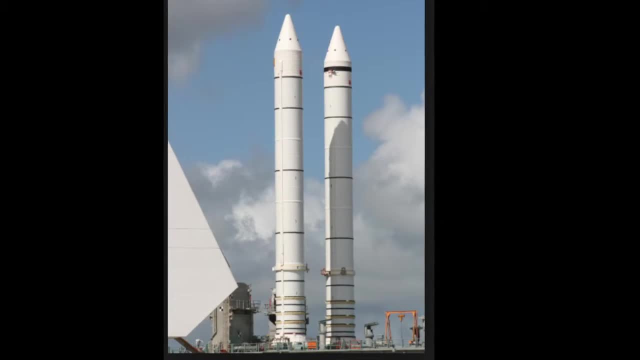 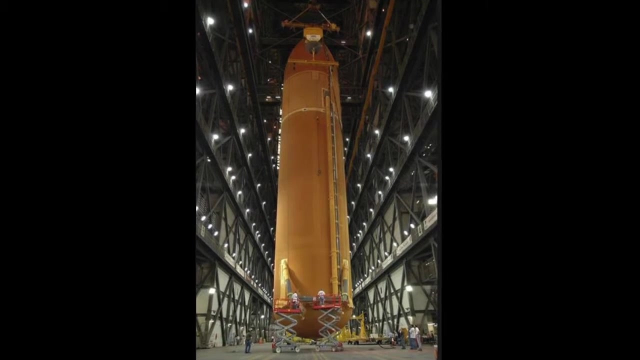 To lift the components. the VAB housed five overhead bridge cranes, including two capable of lifting 325 tons And 136 tons. It was renamed Vehicle Assembly Building after the Apollo program and was used to make the space shuttle orbiters and their solid rocket boosters and the external fuel tanks. 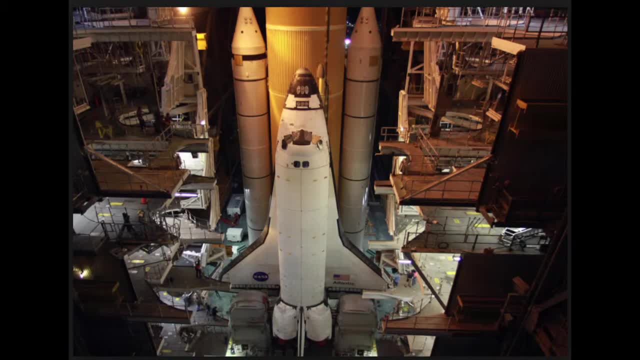 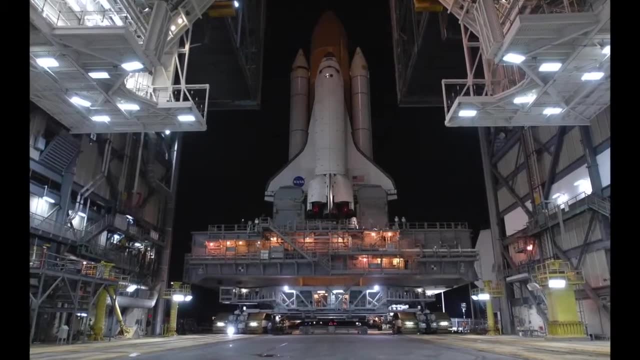 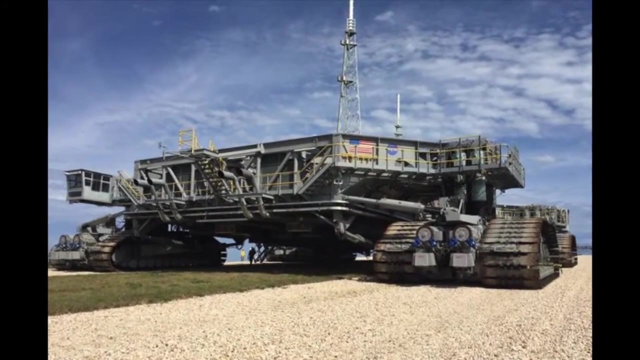 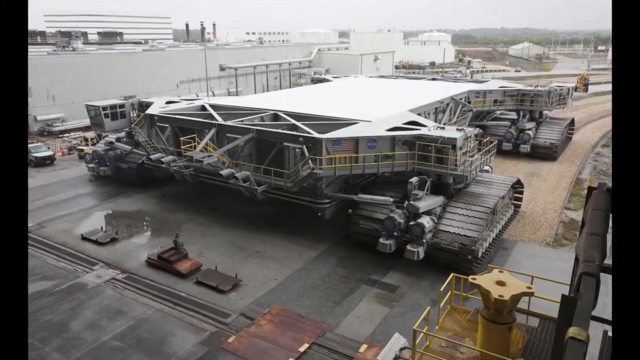 Once assembled, the complete space shuttle transportation system was moved onto the mobile launcher platform and the crawler transporter for transport to the Launch Complex 39, Pad A or B. The crawler transporters are a pair of tracked vehicles used to transport spacecraft from NASA's Vehicle Assembly Building along the crawler way to Launch Complex 39.. 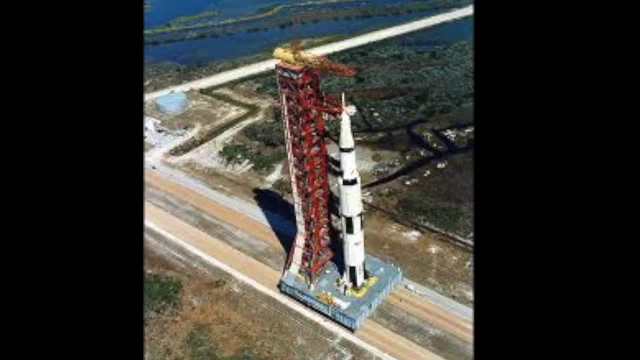 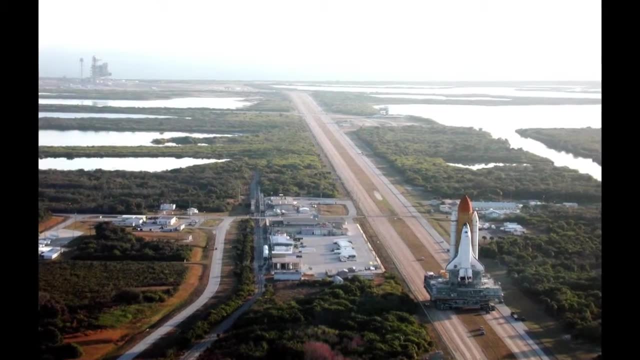 They were originally used to transport the Saturn IB and Saturn V rockets during the Apollo Skylab and Apollo Soyuz programs. They were then used to transport space shuttles from 1981 to 2011.. Thank you for watching and enjoy the rest of your day. 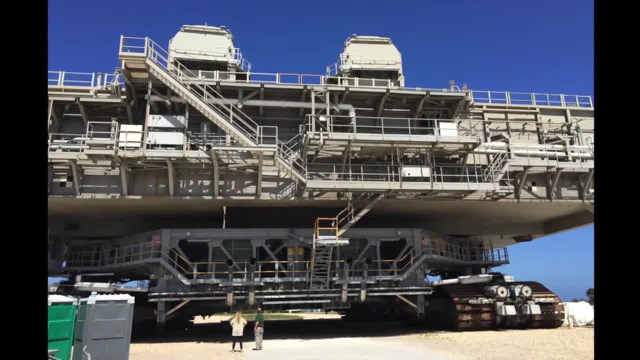 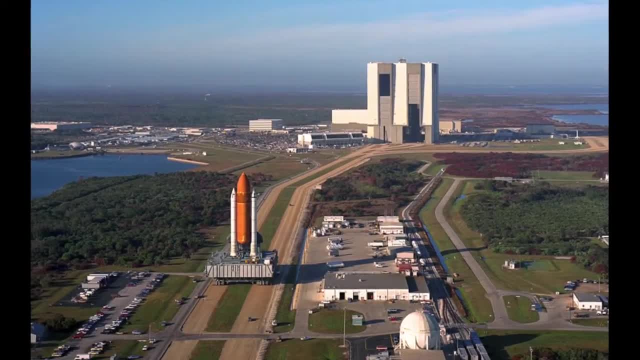 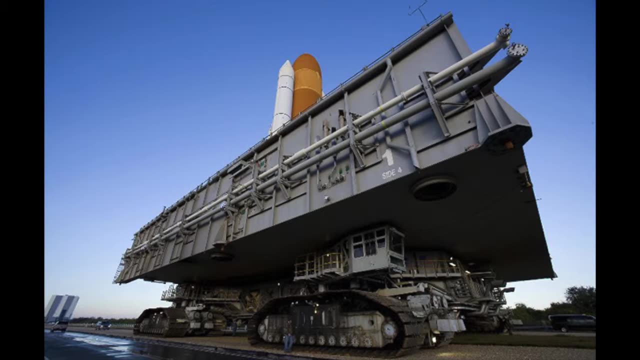 Have a wonderful day. The crawler transporters carry vehicles on the mobile launcher platform and, after each launch, return to the pad to take the platform back to VAB. It takes a team of nearly 30 engineers, technicians and drivers to operate the vehicle. 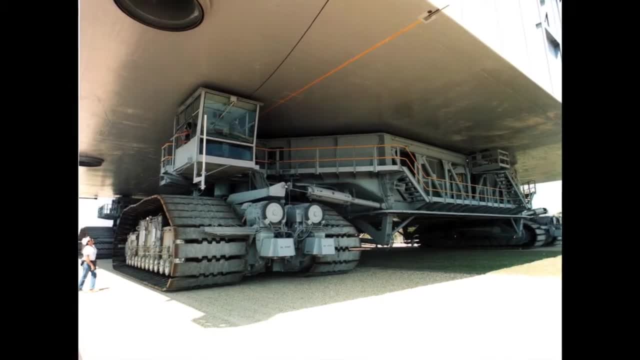 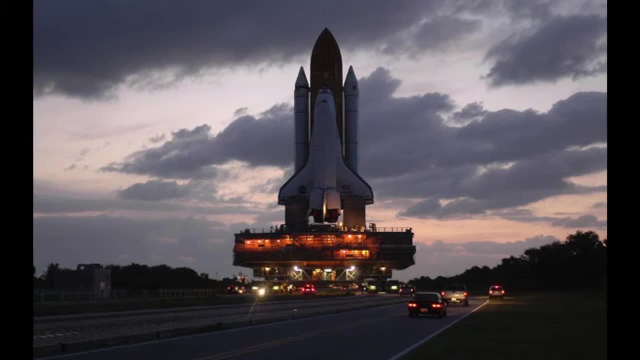 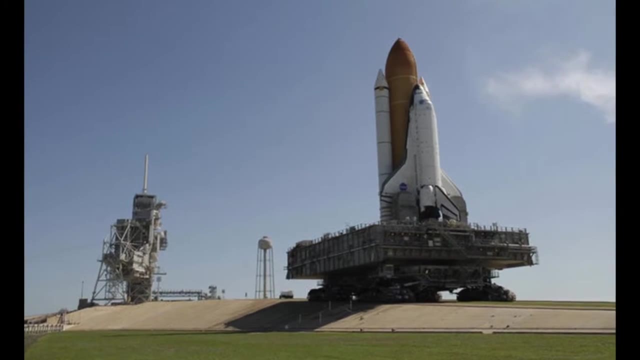 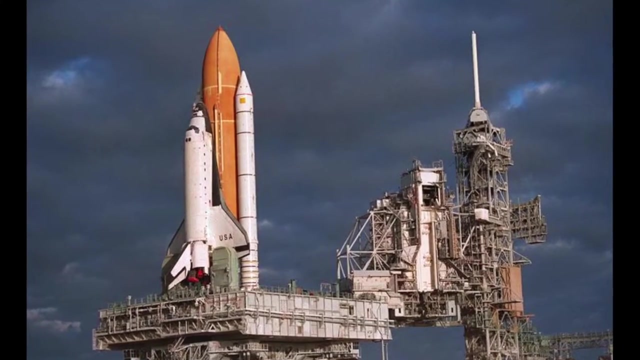 The crawler is controlled from two control cabs located at either end of the vehicle. It travels along the three and a half miles crawler way at a maximum speed of one mile per hour loaded or two miles per hour unloaded. The average trip time from the VAB along the crawler way to the launch pad is about five. 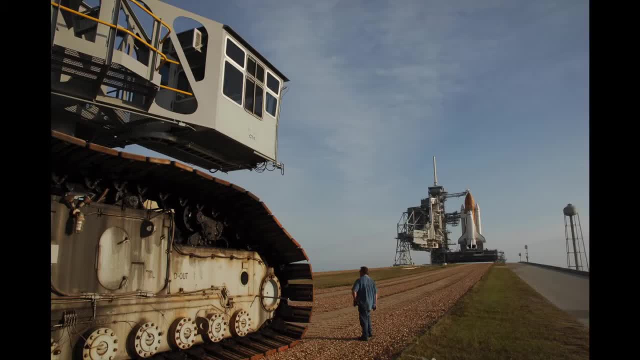 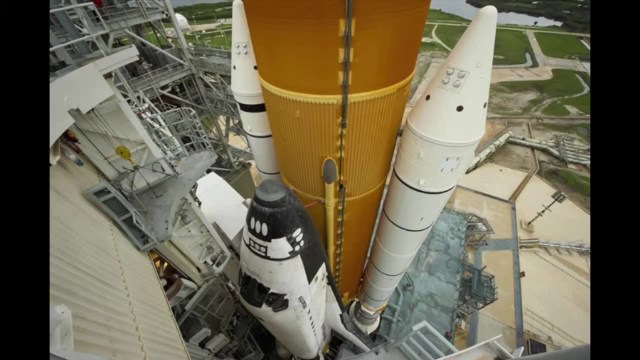 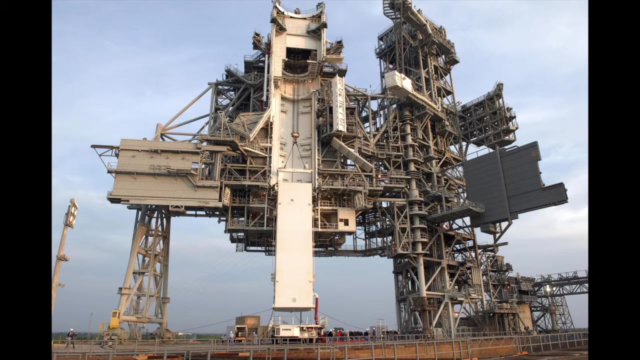 hours. Each crawler way is seven feet deep and covered with Alabama and Tennessee river rocks. The launch towers at each pad contain a two-piece tower. The crawler is equipped with a four-door access system, the fixed service structure and the rotating service structure. 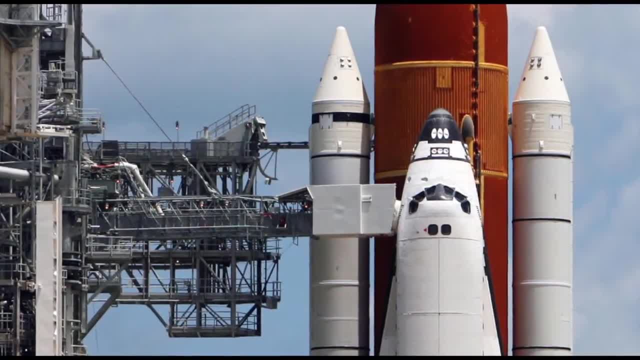 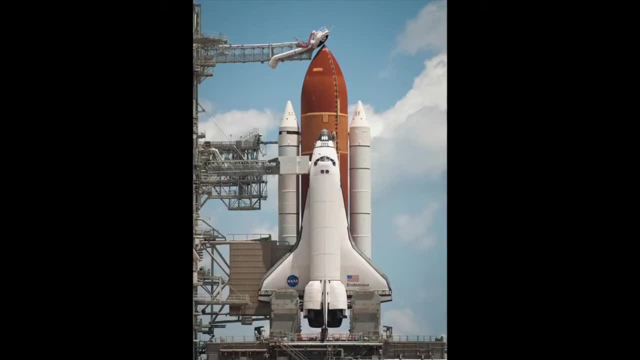 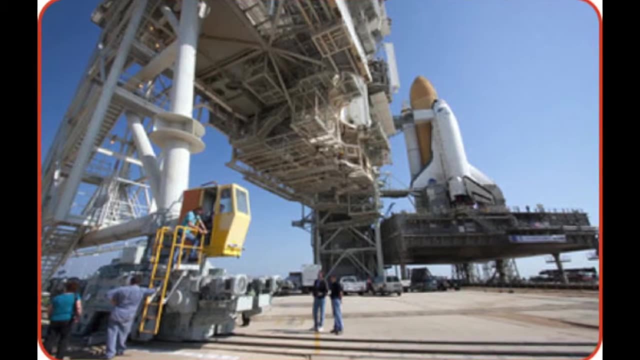 The fixed service structure permitted access to the shuttle via a retractable arm, the white room and a beanie cap to capture vented LOX, the fuels from the external tank. The rotating service structure contained the payload checkout room which covered the payload. 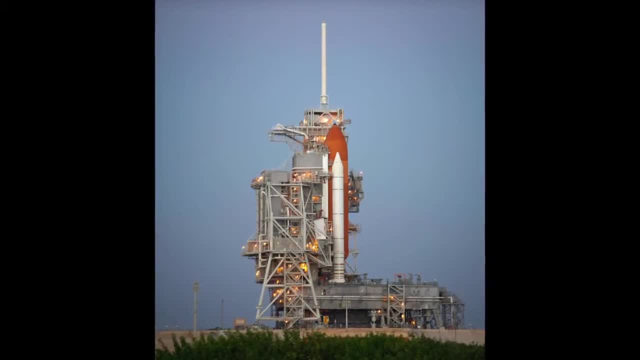 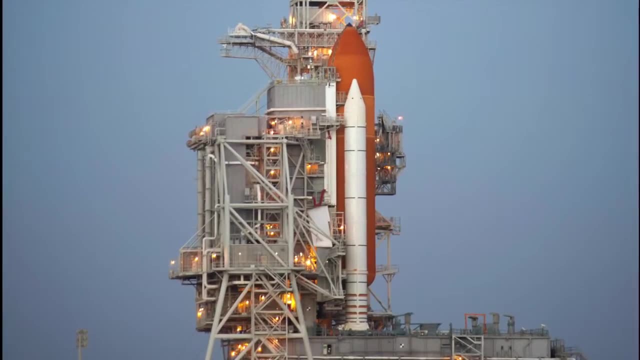 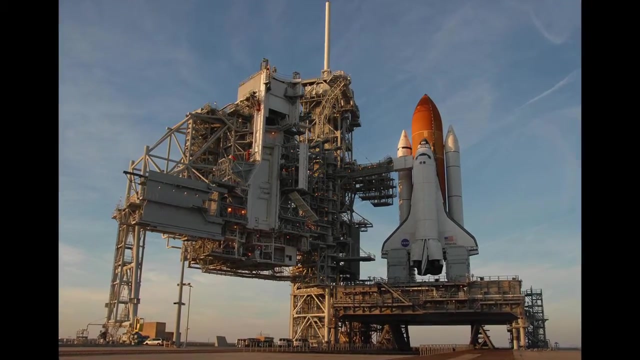 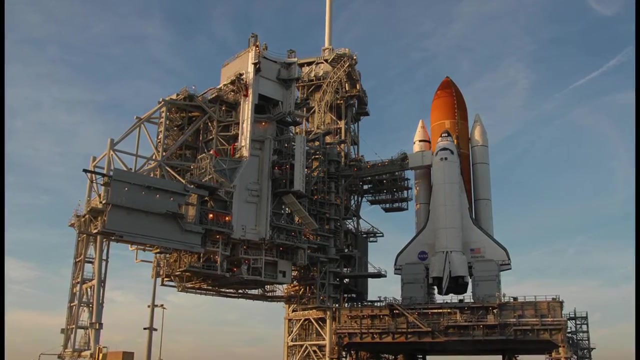 bay and offered clean access to the orbiter. It also protected it from the elements and from winds up to 60 knots. It also provided access for technicians to perform detailed checkout of the vehicle and necessary and biblical connections to the pad. It contained three elevators, two self-propelled platforms and three fixed platforms. 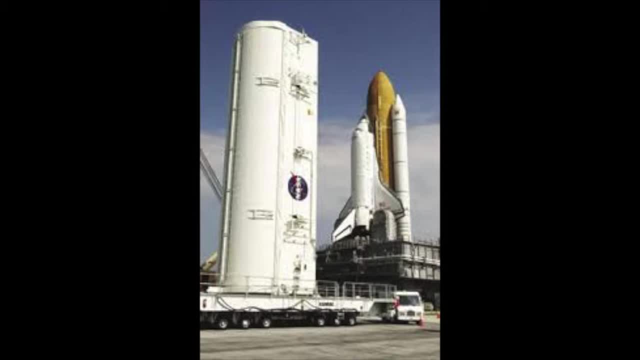 Payloads to be installed at the launch pad are available to the passengers and passengers at the launch pad. Payloads to be installed at the launch pad are available to the passengers at the launch pad. Parallel payloads are 快速取扣, which includes the same payload that are: 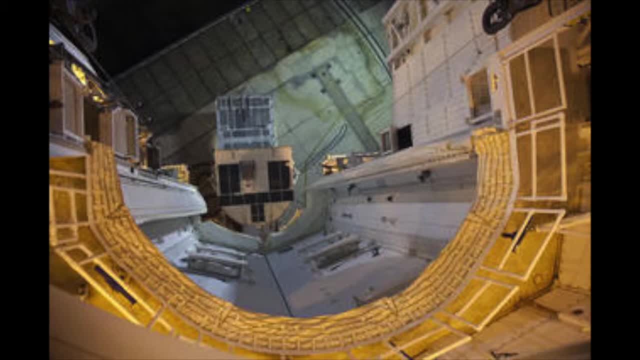 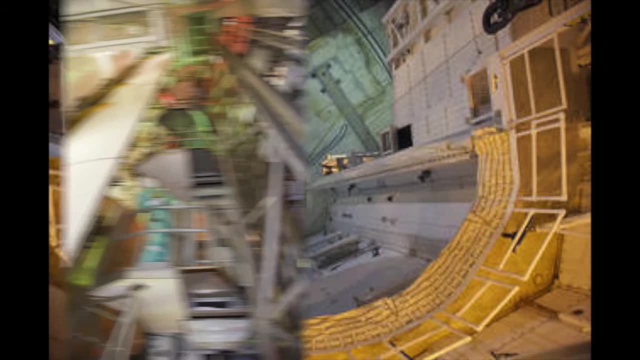 stored in the payloads in the cargo bay. Parallel payloads are supplied to the payload by a vertical transporter, by a special sub-test unit or a single drop to the payload. The payload was then installed vertically at the payload changeout room. Other payloads would have been pre-installed at the orbiter processing facility and transported. 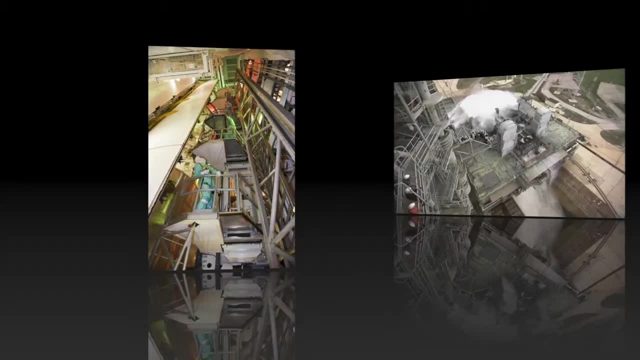 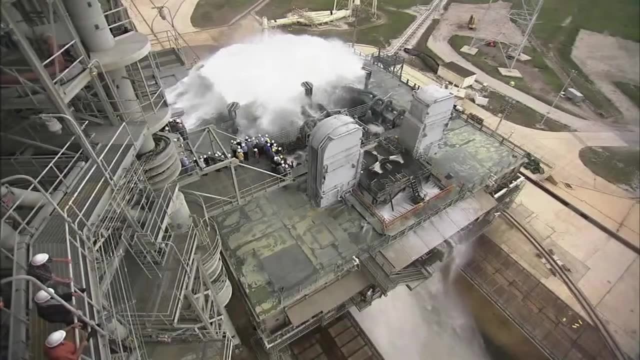 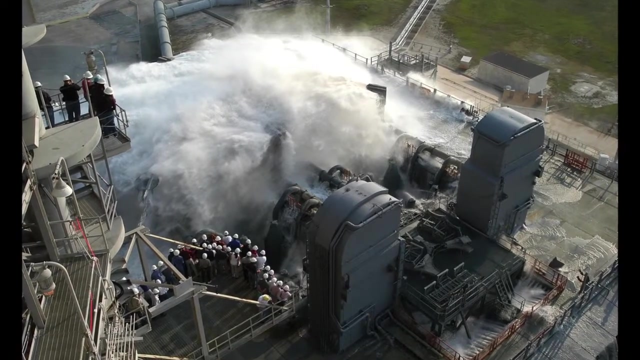 within the orbiter's cargo bay. Also, the payload was used to protect the space shuttle and payload. The payload can be used to easily control the launch pad, which is located to the left of the payload, of the intense sound wave pressure that's generated by its engines: An elevated water. 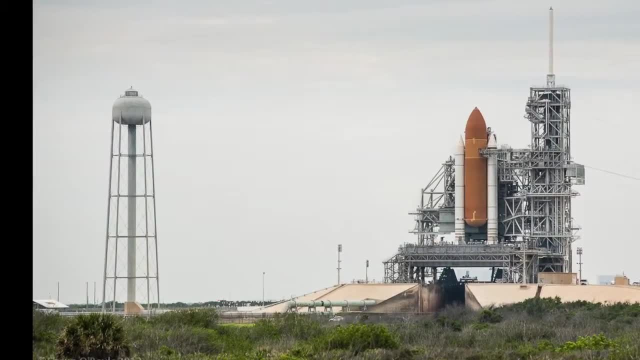 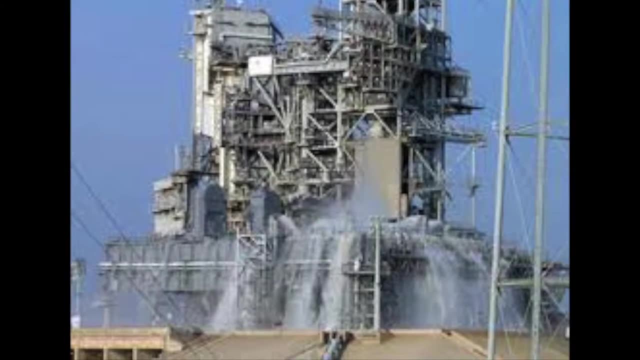 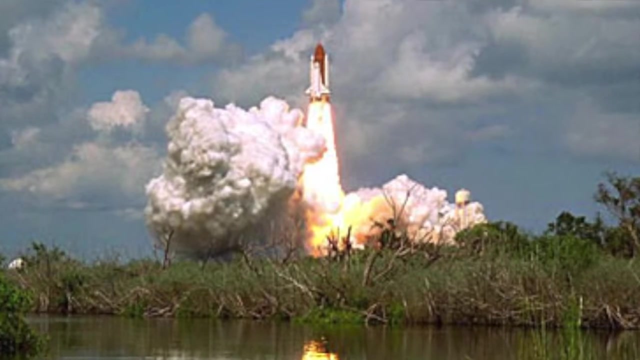 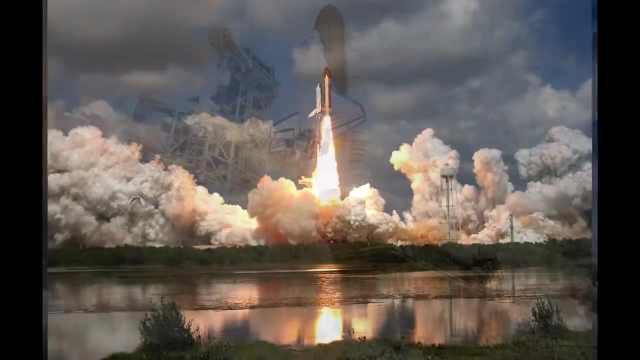 tank is near both pads. It has a 290-foot tower and stores 300,000 gallons of water, which was released onto the mobile launch platform just before engine ignition. The water muffled, the intense sound waves from the engines Due to heating of the water, a large quantity of steam. 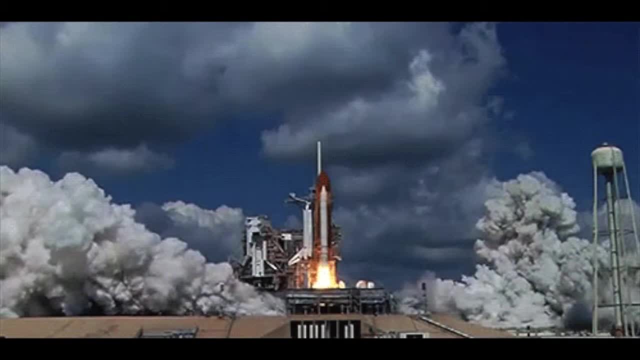 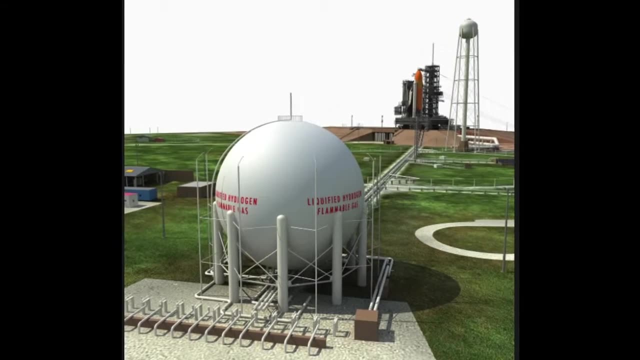 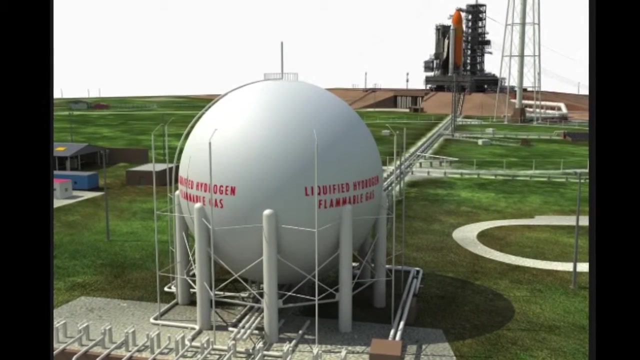 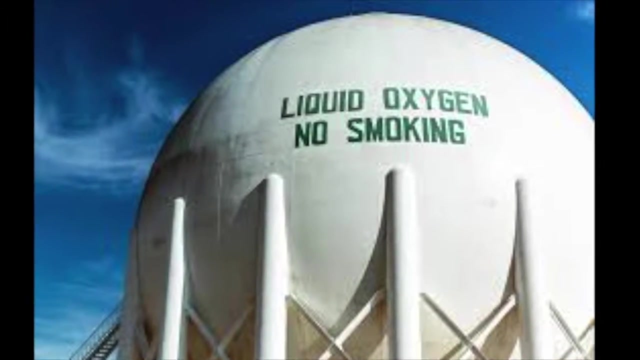 was produced during the launch, not smoke Fueling. the external tank takes place on the pad. The large cryogenic tanks located near the pad store the liquid hydrogen and liquid oxygen LOX. The highly explosive nature of these chemicals require numerous safety measures at the launch complex. The pads are located 8,730 feet away from each other Before. 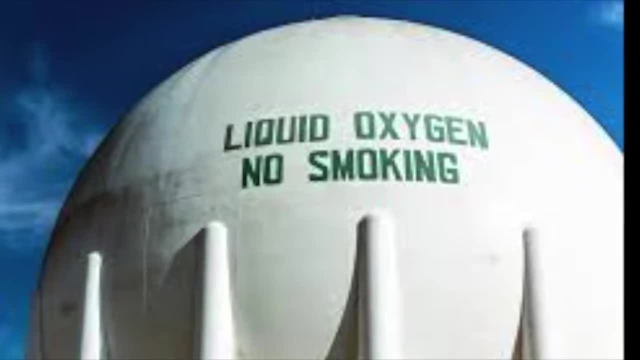 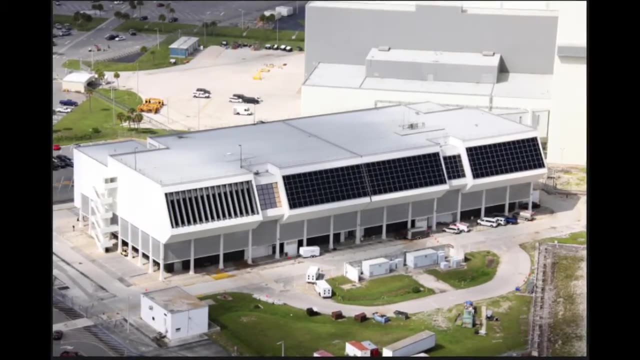 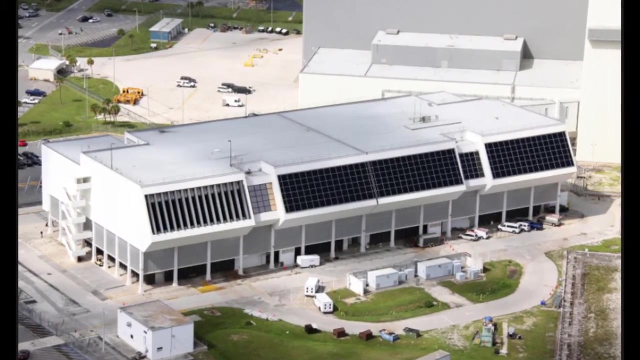 tanking operations began and during launch, non-essential personnel are excluded from the danger area. The four-story launch control center is located three and a half miles away from Pad A, adjacent to the Vehicle Assembly Building. for safety, The third floor has four front. 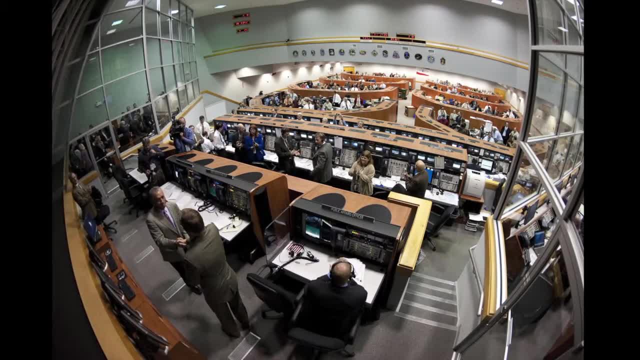 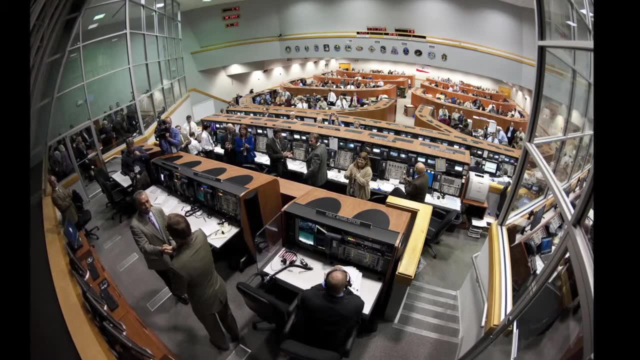 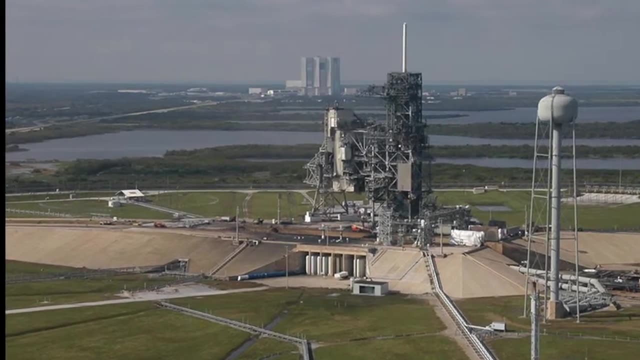 firing rooms, each with 470 sets of control and monitoring equipment. The second floor contains telemetry tracking instrumentation and data reduction computing equipment. The LCC was connected to the mobile launchers by a high-speed data link and, during launch, a system of 62. 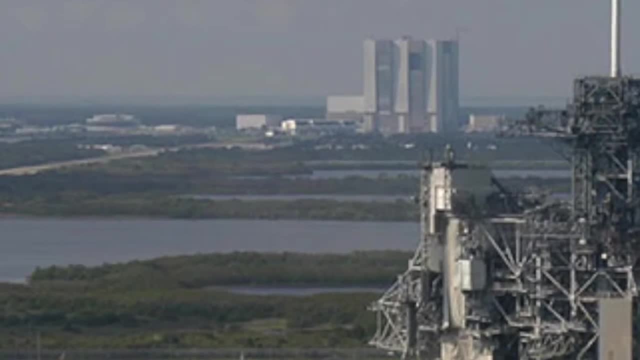 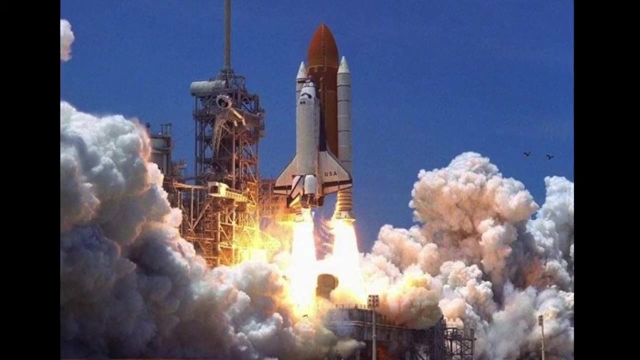 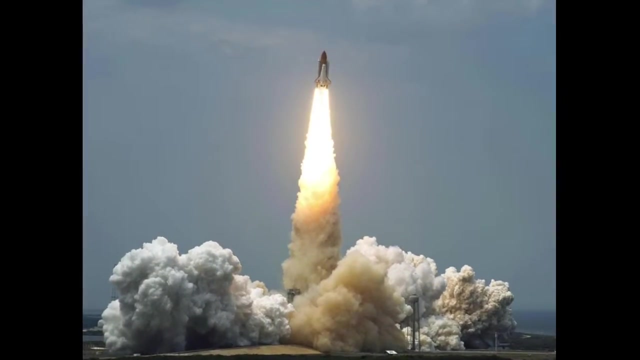 closed-circuit television cameras transmitted to 100 monitor screens in the LCC 3…2…1…LIFT OFF LIFTOFF OF THE SPACE SHETTLE. It takes only 7 seconds for the shuttle to clear the tower and then all controls transfer. 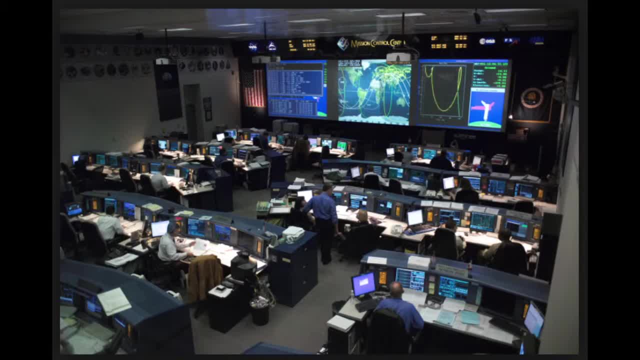 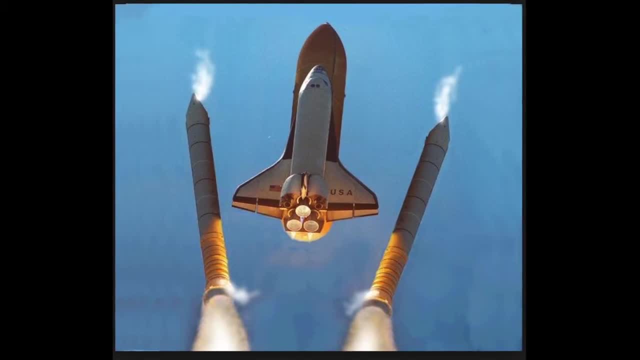 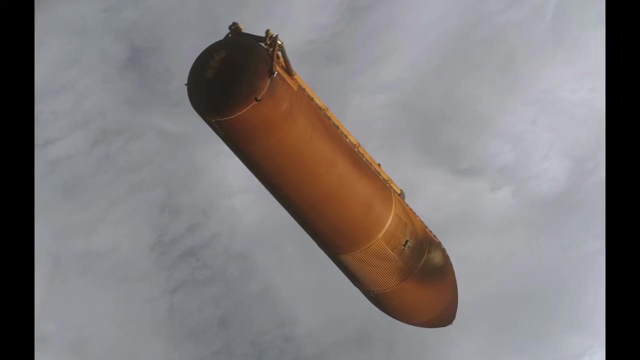 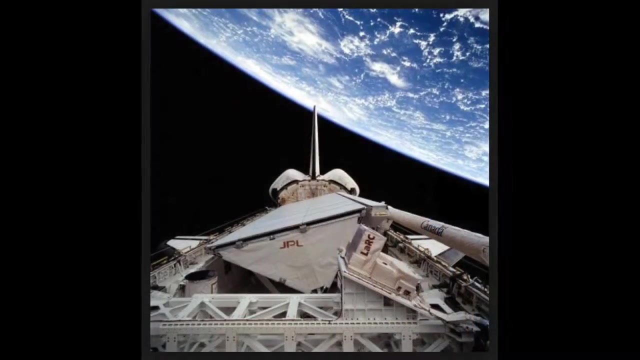 to the Johnson Space Center in Houston, Texas. Two minutes after launch, the solid rocket boosters jettison away from the orbiter and fall back to Earth to be reused. After reaching 17,500 mph, the shuttle jettisons the external tank to fall back and burn up as it enters our atmosphere. 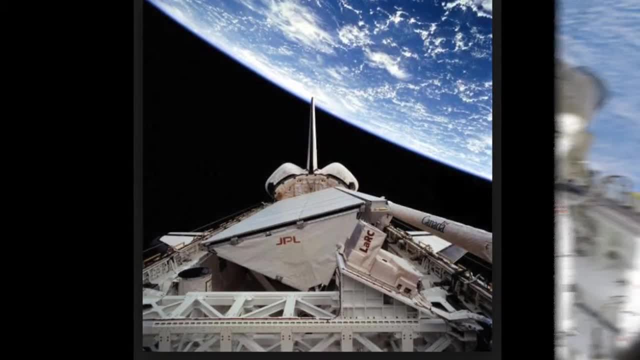 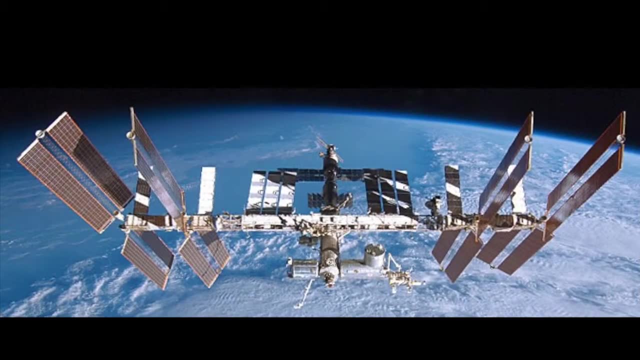 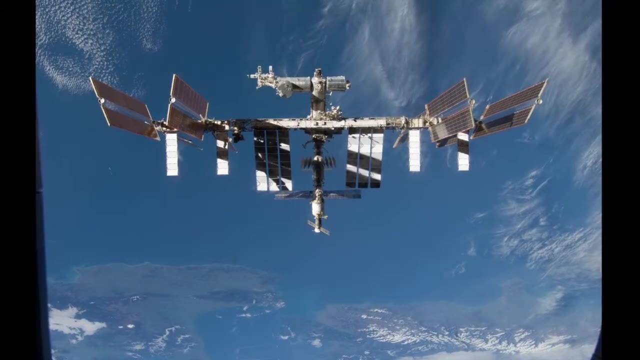 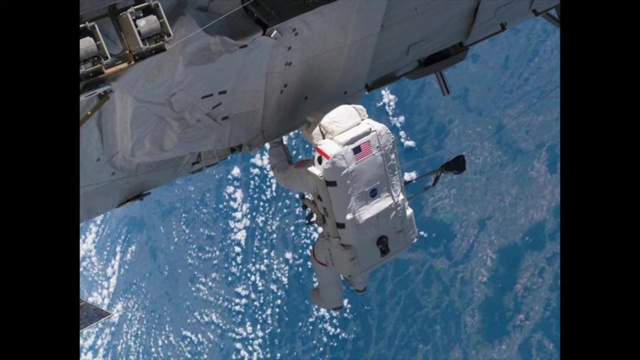 You are now in low Earth orbit. Here the astronauts do their experiments, they do spacewalks and deploy satellites. The astronauts work on the International Space Station and it is the biggest artificial satellite in low Earth orbit. Its first component launched into orbit in 1998 and the ISS is now the largest artificial body in orbit and can often be seen with the naked eye from Earth. 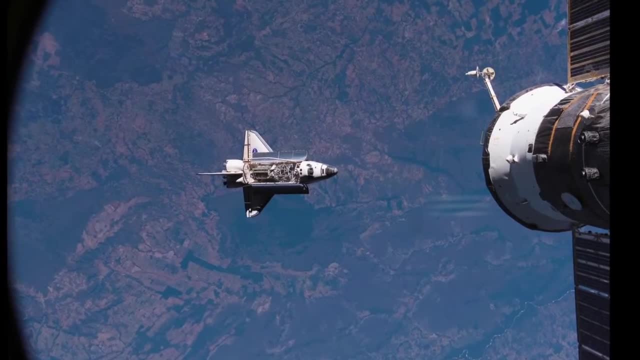 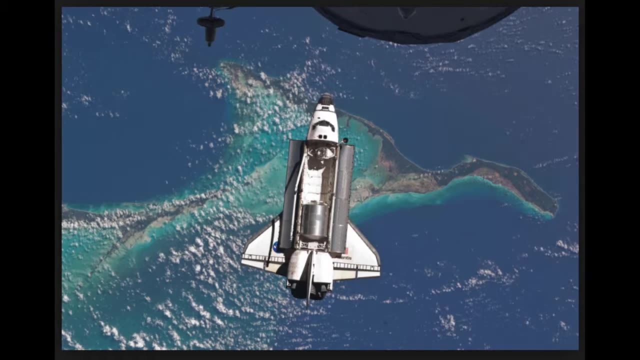 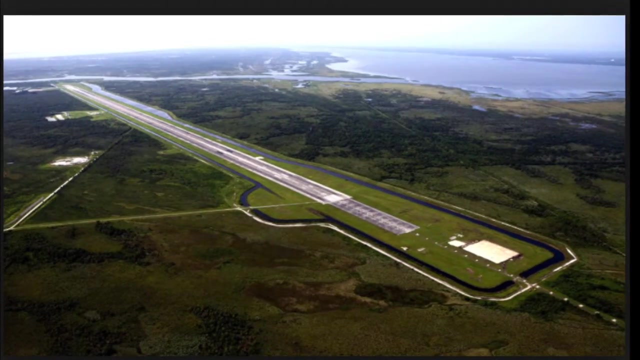 The ISS consists of pressurized modules, external trusses, solar arrays and other components. The ISS components have been launched by Russian Proton and Soyuz rockets, as well as our American space shuttles. The shuttle landing facility is an airport location. 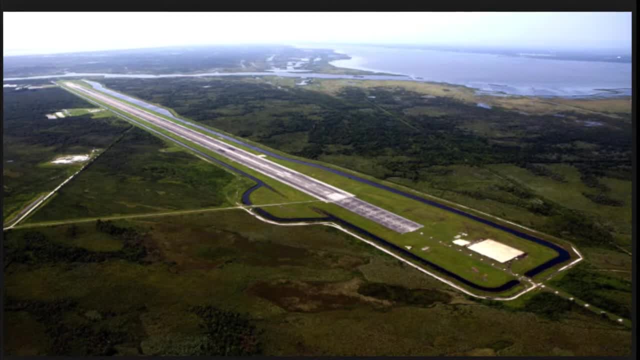 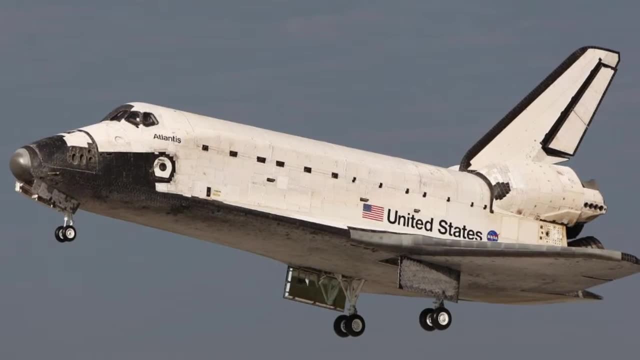 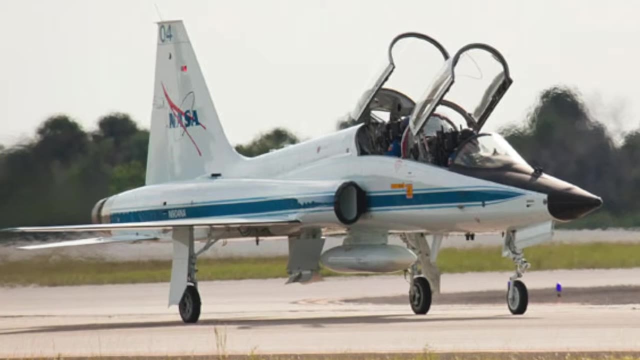 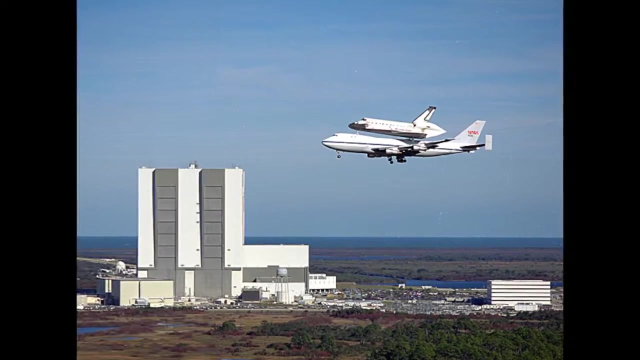 It is located on Merritt Island in Brevard County, Florida. It is a part of Launch Complex 39 at the Kennedy Space Center and was used by NASA's Space Shuttle for landing until the program's end in 2011.. As well as for takeoffs and landings for NASA's training jets and civilian aircraft such as the Shuttle Carrier Aircraft. 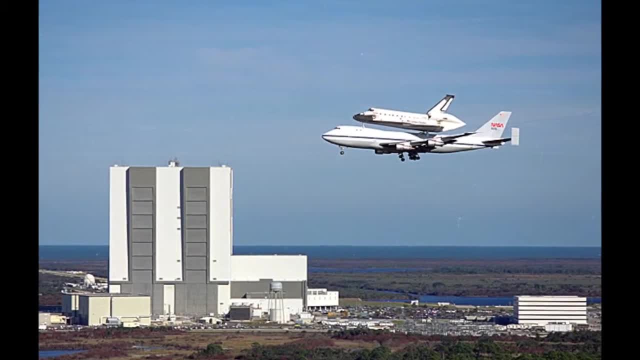 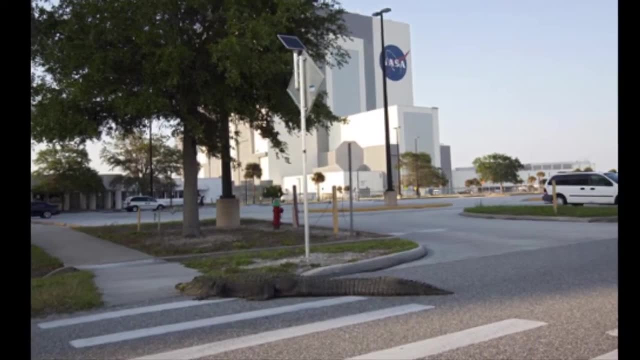 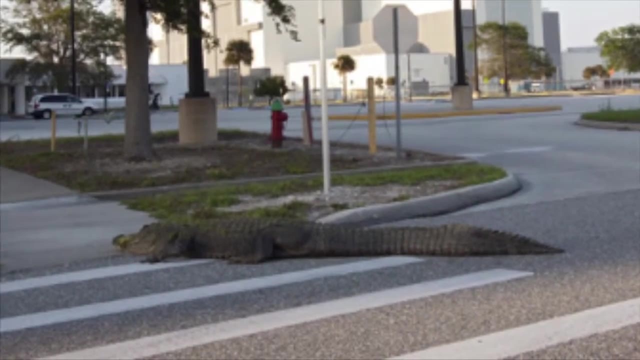 A local nickname for the runway is the Gator Tanning Runway. The shuttle landing facility has some of the 4,000 Gators living at the Kennedy Space Center regularly bask in the sun on the runway. The shuttle landing facility covers 500 acres and has a single runway. 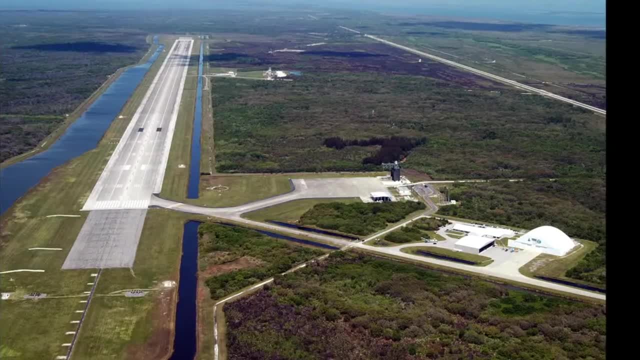 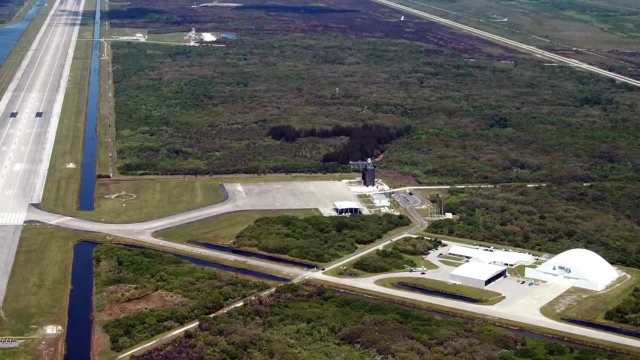 It is one of the largest runways in the world at 15,000 feet, and is 300 feet wide. Additionally, the shuttle landing facility has another 1,000-foot runway. It has another 1,000-foot of paved overrun at each end.